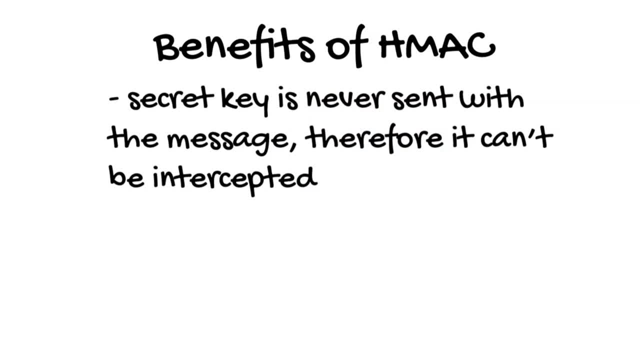 to a password. It is very important to keep the secret key safe. since it is used like a password, it needs to be saved in an encrypted storage. It's also important to use a sufficiently long secret key that cannot be brute-forced by password breakers. Second, an HMAC is based not only on the 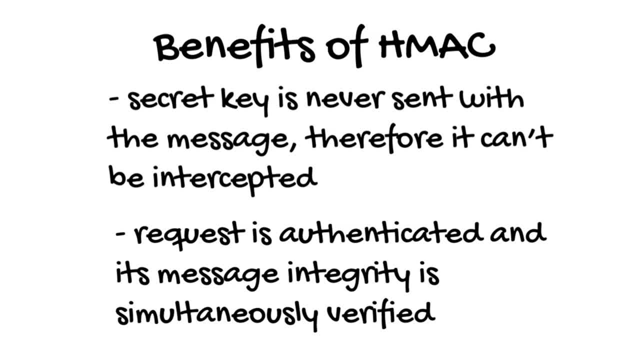 secret key, but also on the message itself. If two HMACs are created with the same secret key but different messages, the resulting code will be different. When the API sees that its HMAC matches the HMAC in the request, it knows the request was not modified during transport. 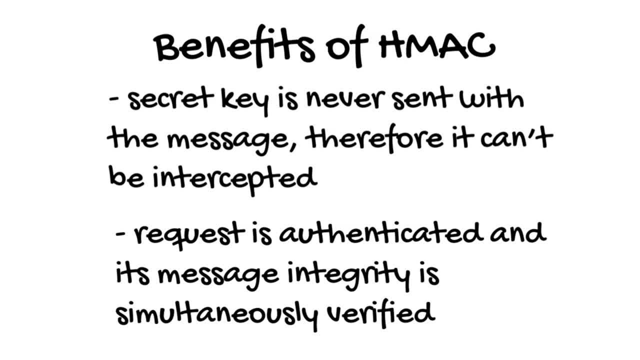 Since hackers will try to hack the HMAC, it will not be able to hack the HMAC To modify messages in between clients and servers. HMAC signatures can be a powerful tool to verify authenticity of requests. I cloned repository node API starter from my GitHub. 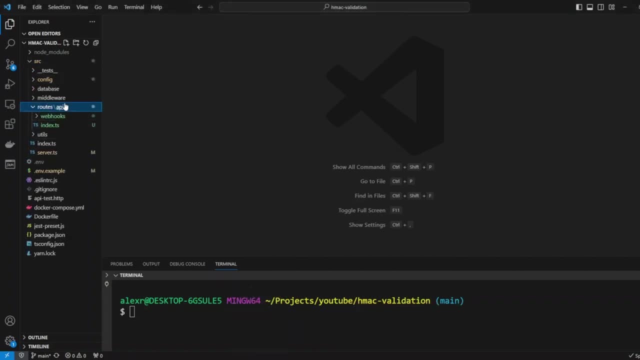 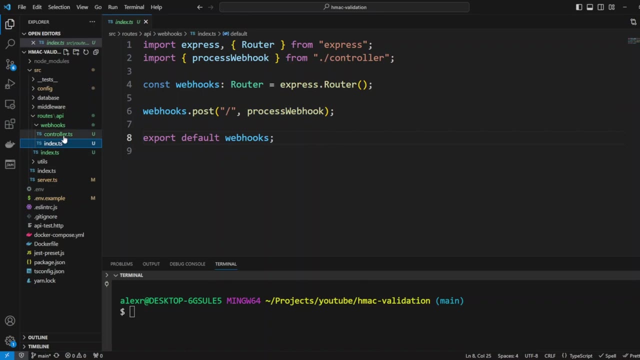 I also created a route in the routes folder API webhooks. And here I have an index file that will use process webhook from the controller. And in the controller we just return OK to the server. And here I have an index file that will use process webhook from the controller. 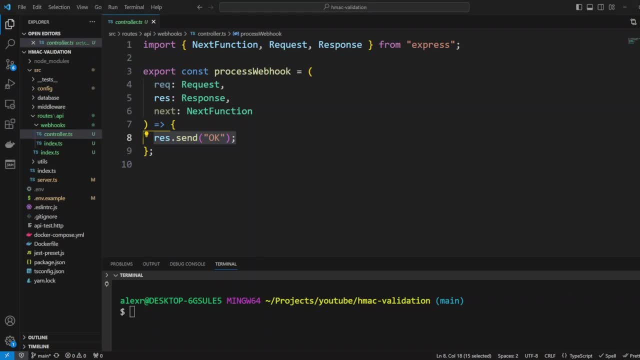 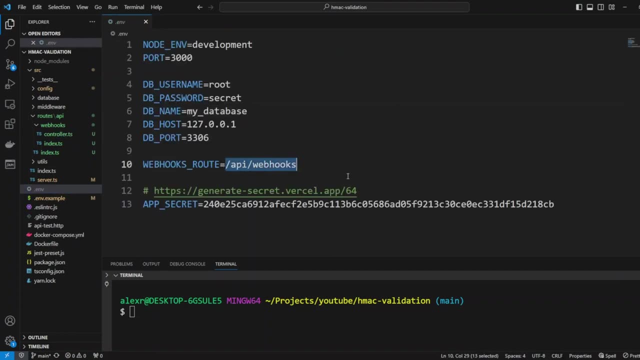 Next, I also added couple ENV variables. In the env file I put webhook routes And this will be API webhooks And I also added app secret variable And I generated secret from generate secretvercelapp And I put as a 64-bit so it's sufficiently long secret. I also updated ENV manager. 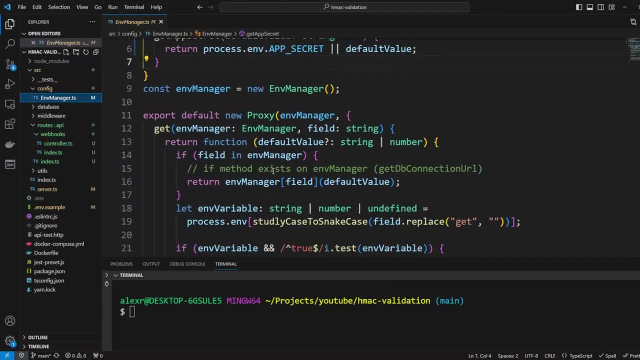 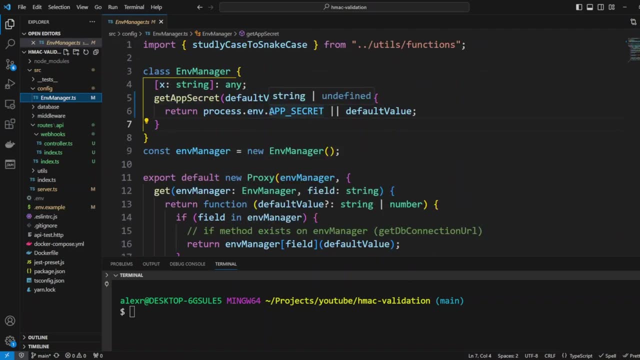 in the config folder And I added secret from generate secretvercelapp And I put as a 64-bit, so it's sufficiently long secret, And I added secret from generate secretvercelapp And I added the function that is called get app secret And this function is returning app secret ENV variable. 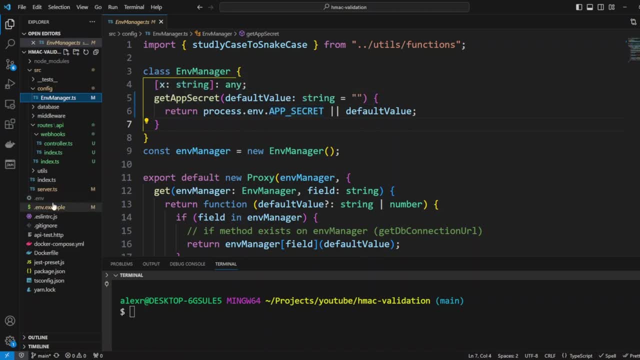 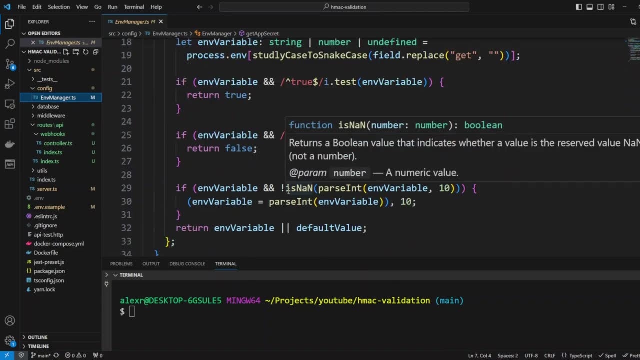 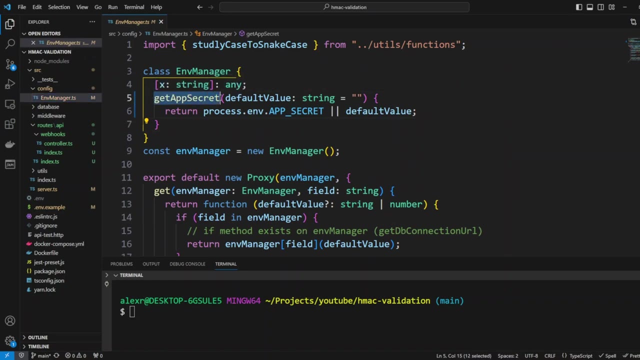 The reason I created a specific function for it is that app secret starts with the numbers, So according to the code in the ENV manager, it will treat it as a number. So in order for it not to convert it into a number, I created a special function for it. Now let's go ahead and test it. 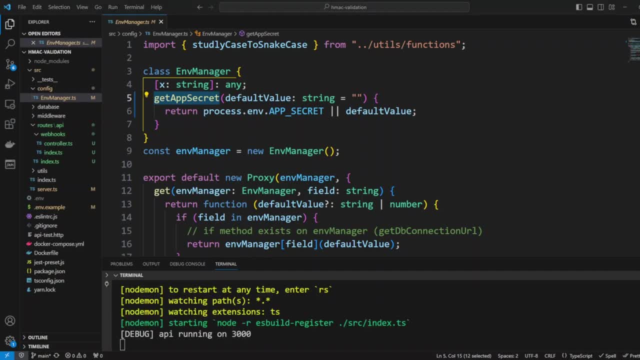 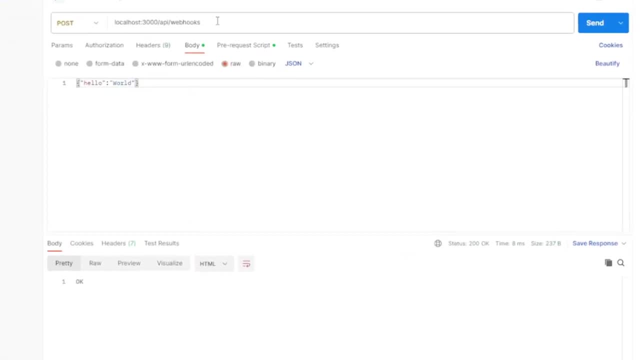 To test our setup, we'll do yarn dev And we will use Postman to make an API call. In a Postman, we will do a post request to API webhooks endpoint And let's click send And we can see that the response is OK- 200.. Now let's go ahead and implement HMAC verification. 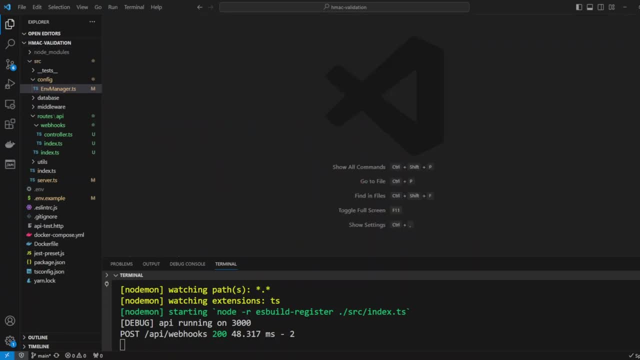 In order to calculate HMAC, we need to get hold of raw body of the request. The easiest way- do it in express- is to use verify function in express json middleware. let's do exactly that. let's go to serverts function and in expressjson let's put the following code: 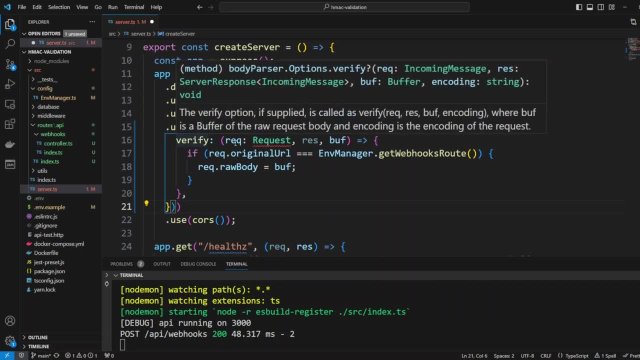 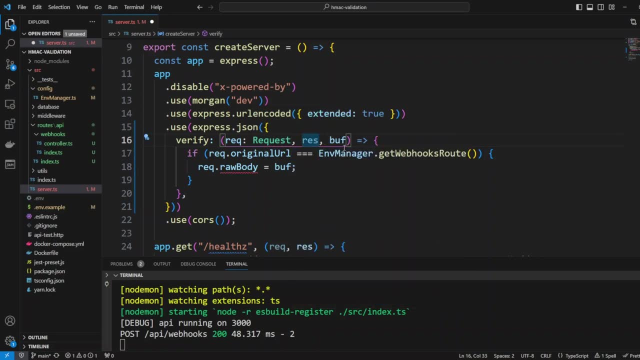 we're going to be using verify function and we're going to take request, which is the request from express, and it will take response and the buffer. so we will check if the request of the original url is the webhooks route and then we assign buffer to request raw body property. 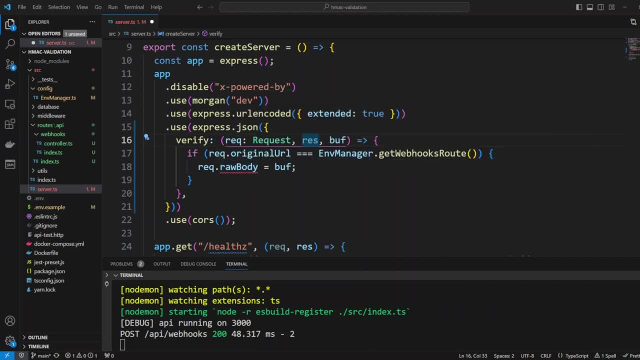 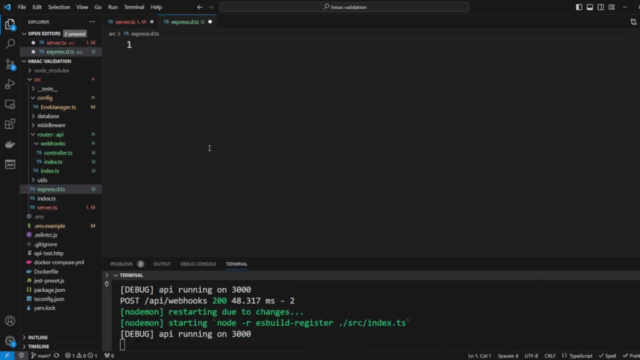 however, this property does not exist on express request and this is why typescript complains. we need to add a raw body property to express request interface. in the src folder let's create a new file, expressdts. that will be a declaration file, and we will put the following code in there: we will import express, then we're going to declare. 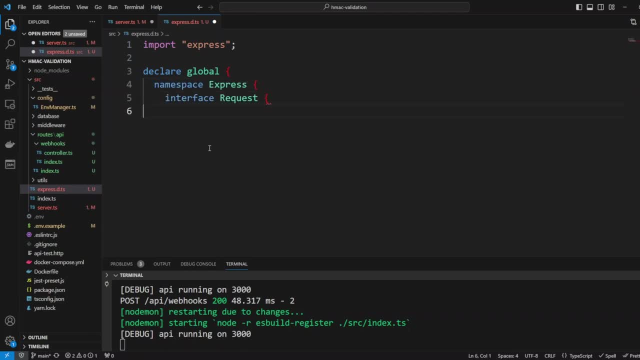 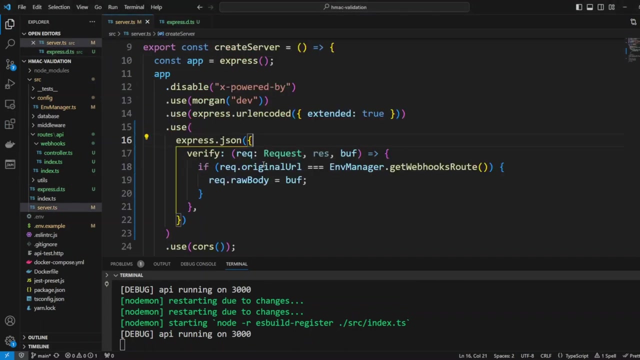 global namespace express. this is how express has it. then we're going to use take the interface request and we add a raw body optional property. that will be a type of buffer, and that's it. let's go ahead and save our changes. and now, if we go back to serverts, file. 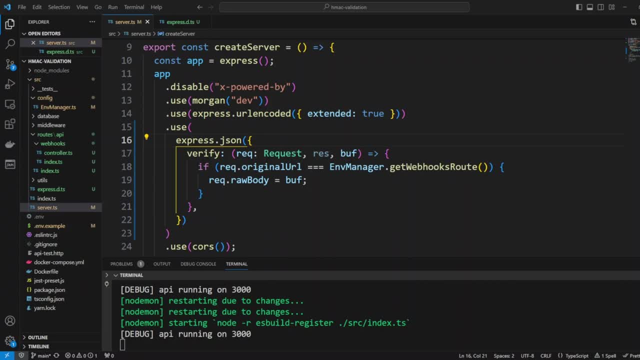 typescript is happy, since interface declarations get merged. we essentially extended express request interface by adding raw body property. we also have to be sure that the expressdts file is included into types option of the tsconfigjson. if you have a types option and they allow the show folder where you add physical stuff, that is Carmenllo. 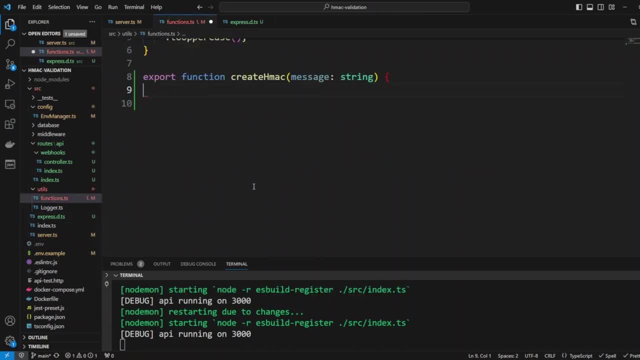 we have a tab feature that we call srax and it didn't need any time at all. we wy only add the text that we're going to put on here and we imported it to srcdems. now we will have to create a SPAND exhibition intro that will be called space for more specific prosperity. 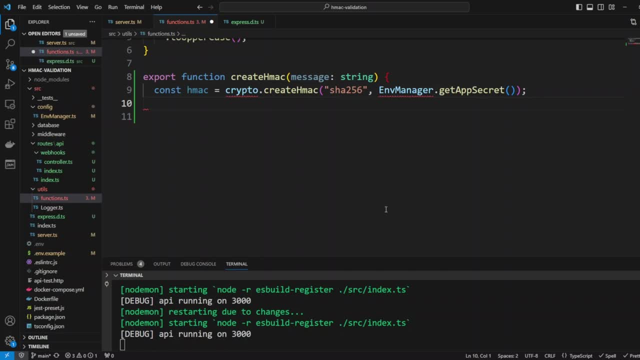 versions like wellness space. next, there will need to be an example display default web following changes. basically, we'll make it our personal menu of the channel and we'll make it that you're getting lots and lots of different지는. we'll execute digest and we'll use a hexadecimal. the next function will be verify HMAC and we'll take 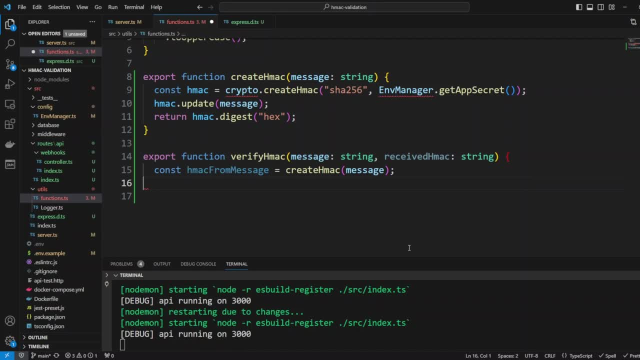 message and it will take received HMAC and again, we're going to be calculating HMAC from this message and we'll use the function create HMAC that we just wrote and we will return crypto timing safe equal and we'll take buffer from HMAC from message in the UTF and we'll take buffer from 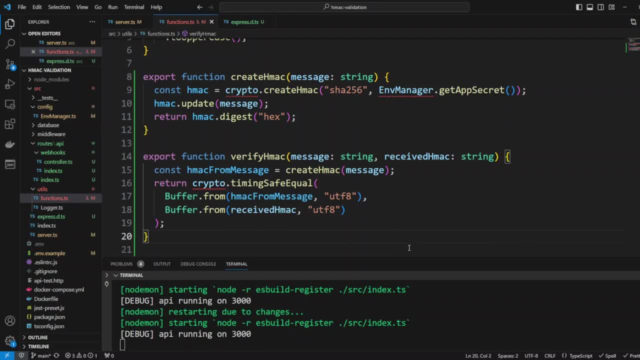 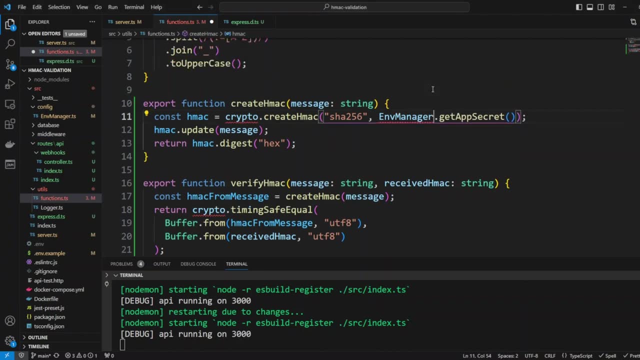 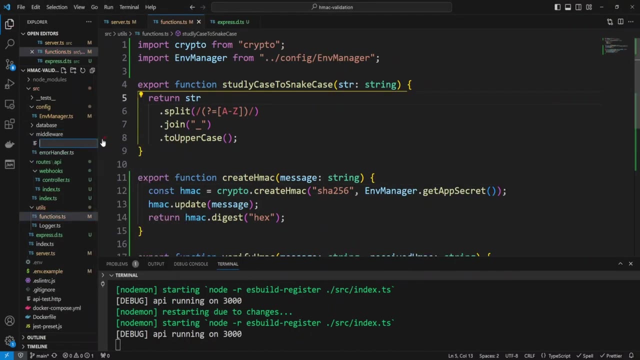 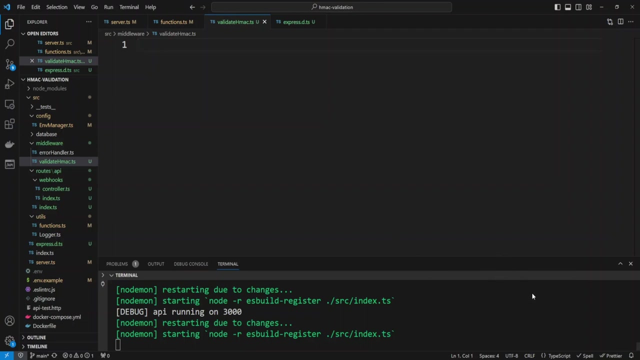 received HMAC and the result will be: either they're the same or different. now let's also not to forget to import in the manager and also crypto. now let's create new file in middleware folder. we'll call it validate HMAC and let's write the code that will validate the incoming HMAC. 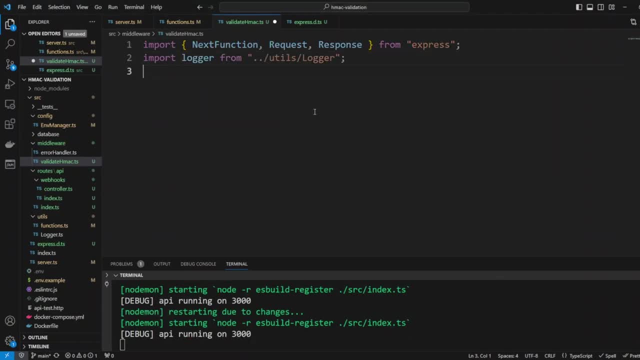 first let's import next function request any response from express and also log logger from utils logger and import verify HMAC from utils functions. so we're going to export default function validate HMAC, we'll take request response and next we're gonna get HMAC signature and we will get it from x HMAC header and if there is no x HMAC header, hence there is no HMAC. 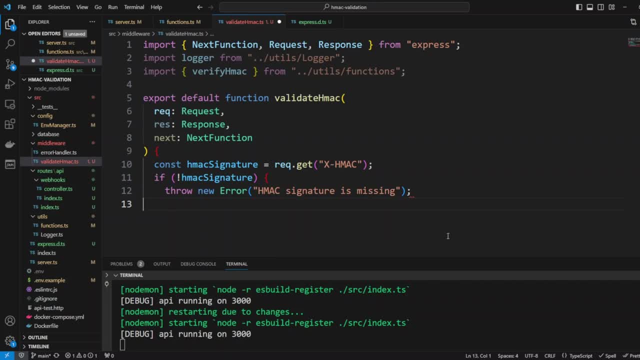 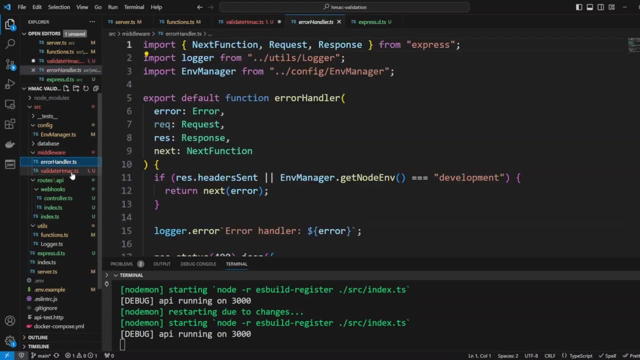 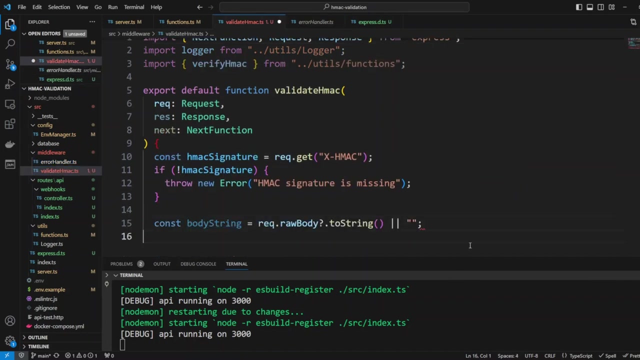 signature, we'll throw a new error: HMAC signature is missing. this error will be caught in the error handler middleware. so that's why we're going to be just throwing errors in the validate HMAC. so next we're gonna create a body string. we will take the request row body and put. 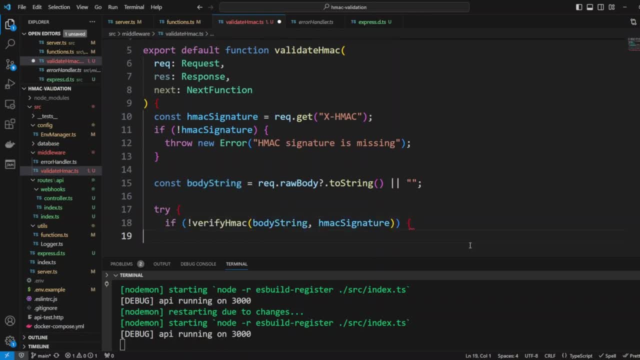 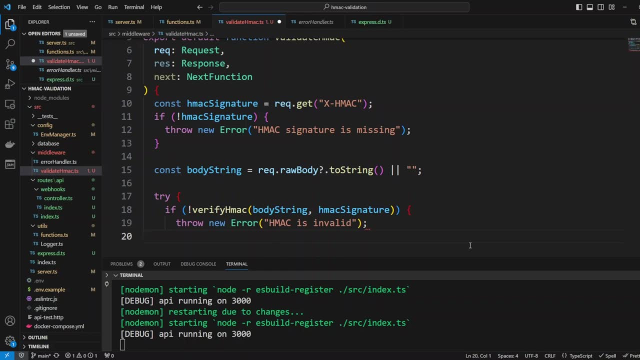 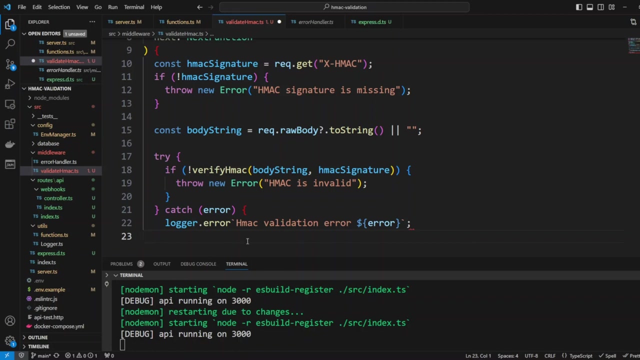 it to string because it's a buffer, and then we're gonna try to verify HMAC and if HMAC doesn't- is not very verified- we'll throw an error. HMAC isn't valid, then we're gonna. we're gonna also have the page block, because verify HMAC function can also throw an error to us, and then we're gonna log that. 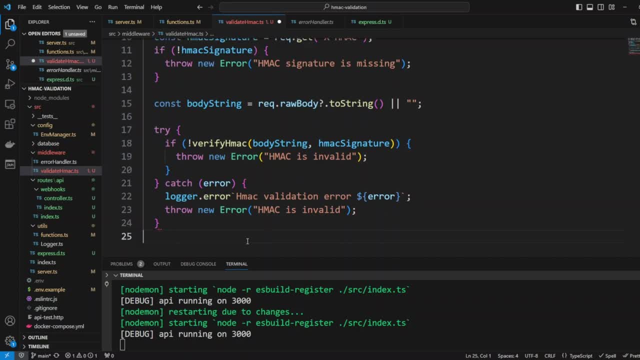 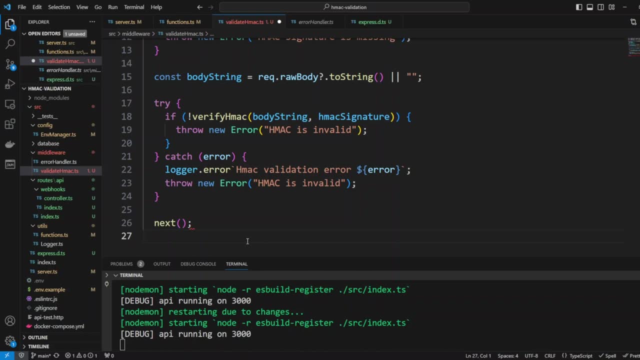 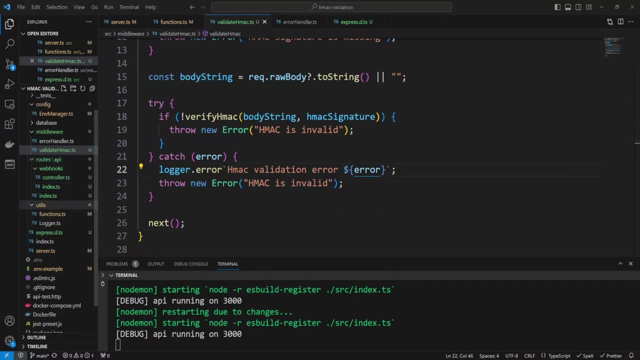 error and throw it so error handler can catch it, and after that we'll just put next function. if everything goes through and HMAC is verified, we'll pass the request to the next function. and finally, let's attach this middleware to the webhooks route. let's go into the indexts file in. 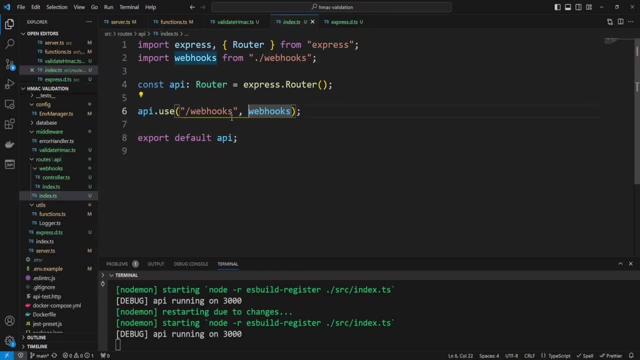 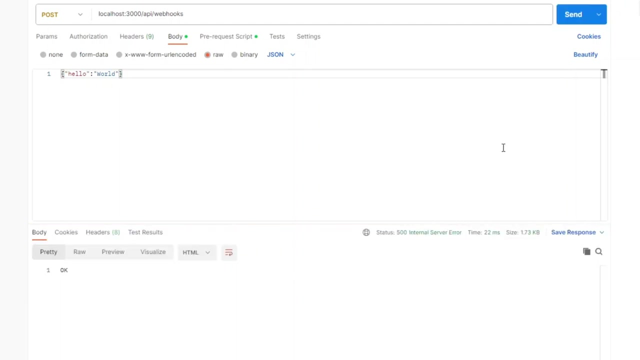 the API folder and right after the webhooks route, we'll just put our validate HMAC middleware, and we also need not to forget to import it. now let's go ahead and make an API request in postman, let's go ahead and click send again and, as a result, we have an error. the reason why it's showing like: 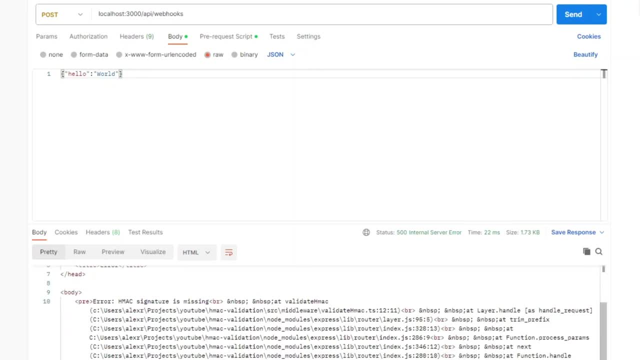 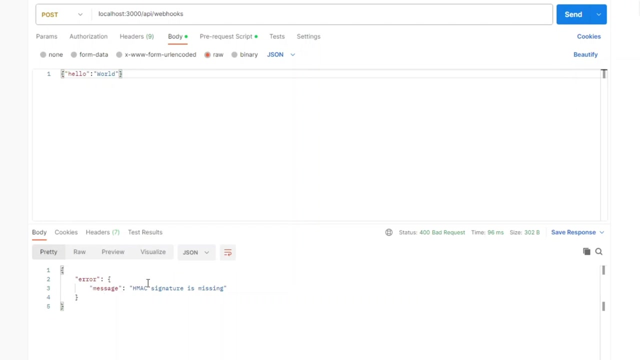 that is because the application in the development environment, so for developers it's going to be easy to see it. let's go ahead and change the environment to production. and now we got the error message: the HMAC signature is missing. the reason it says that is because we do not have X HMAC header and the value for it. so let's create it. we'll put. 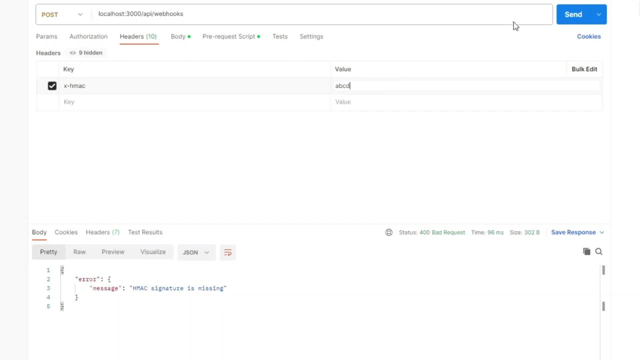 X HMAC and put ABCD. now, if we click send, the response will be that HMAC is invalid. in order for each Mac to get validated, it needs to be created on the client in the same way it was created in the server. so we can simulate that in postman by using pre-request script. let's uncheck. 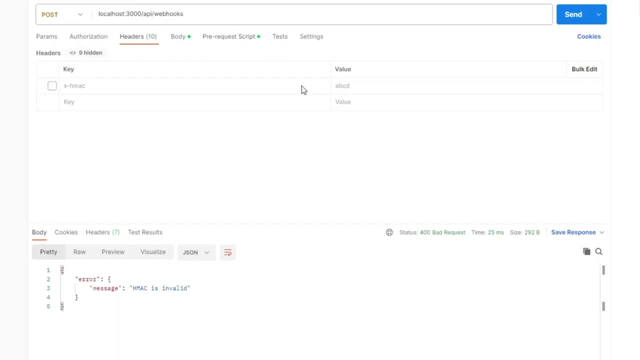 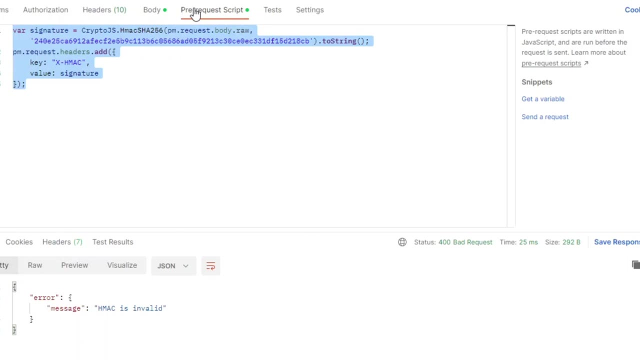 H, H, HMAC header here and just go to pre-request script. in the pre-request script we're going to put the following code: we're going to calculate the signature using SHA 256, the algorithm, and we're going to get the raw body and we will use the same key and then we put it to.